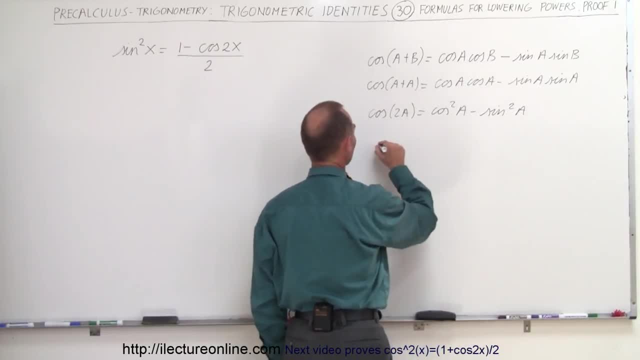 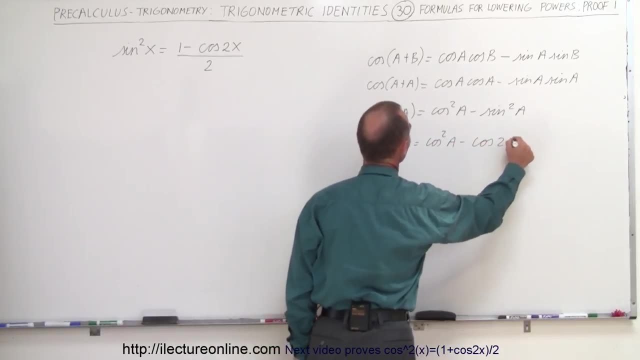 oh, not the cosine. I want to move the sine over here. so the sine squared of a is equal to the cosine squared of a minus the cosine of 2a. Now we're starting to move the cosine squared of a. We're going to make this look a little bit like here. 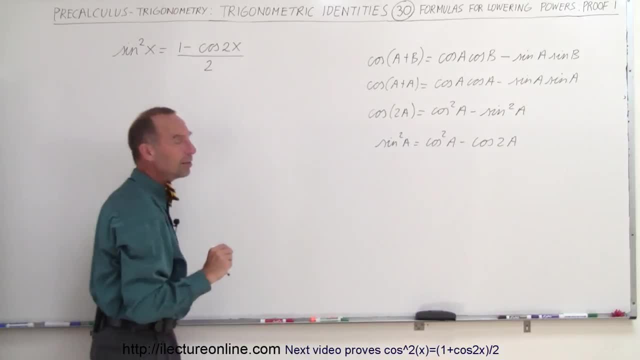 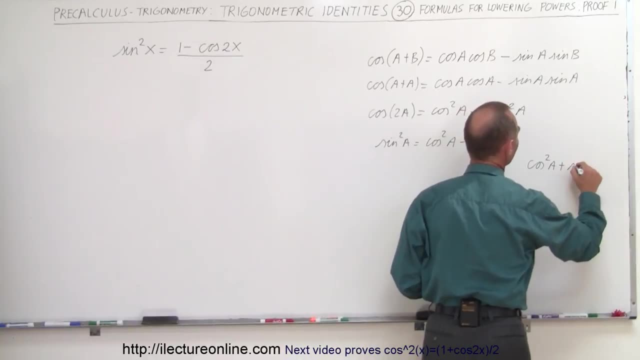 We already have the sine squared. We have the cosine of 2 times the angle. Now we have to make one more change. Remember that the cosine squared of a plus the sine squared of a is equal to 1, which means that the cosine squared of a can be written. the cosine squared of a can be written as 1 minus the sine squared of a. 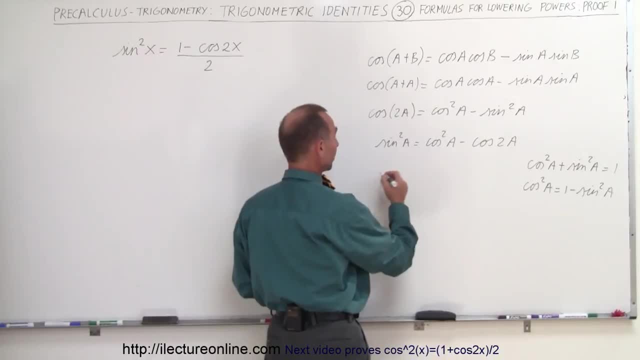 So if you make that substitution into this equation, we get the following thing: We get: the sine squared of a is equal to. instead of this, we're going to write that 1 minus the sine squared of a minus the cosine of 2a. 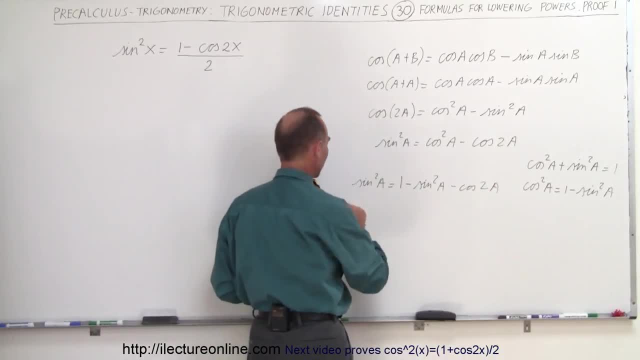 And now we're going to move the sine squared of a to the left side. So now we have the sine squared of a plus the sine squared of a is equal to 1 minus the cosine of 2a, And I think now you can start seeing the resemblance between this and that. 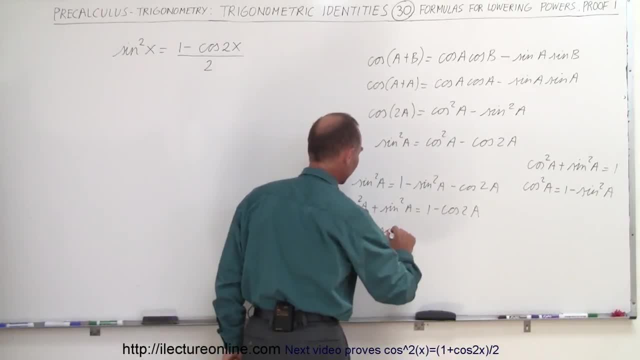 We're going to add these together, So now we have 2 times the sine squared of a. The sine squared of a is equal to better square 1 minus the cosine of 2a, And then if we divide both sides by 2,, 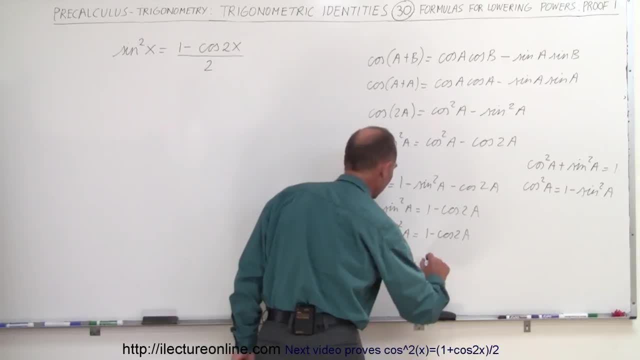 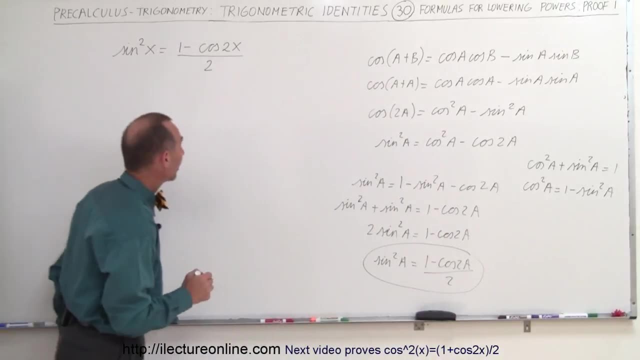 we get: the sine squared of a is equal to 1 minus the cosine of 2a all divided by 2.. And that's the formula that we have over here. It looks exactly the same, except we used x instead of a. 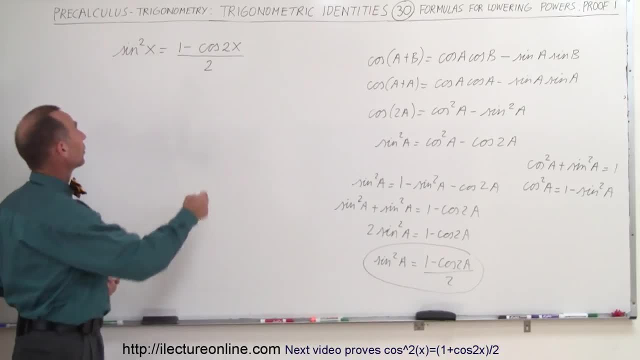 And of course, that's the formula that we used to lower the power of one of the sines for the sine function. The cosine function in this case is for the sine function. In the next video I'll show you how we got the equivalent equation for the cosine squared of a. 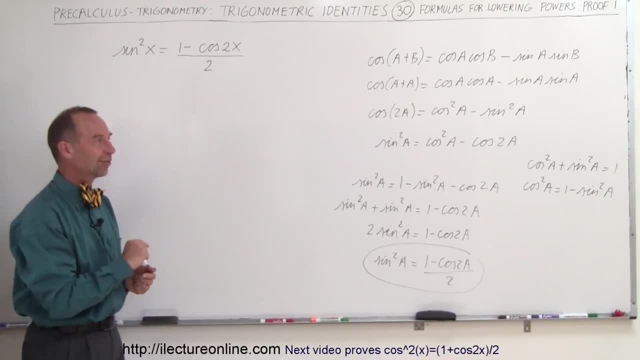 Again, similar kind of approach. So if you'd like to see that, stay tuned for the next video.